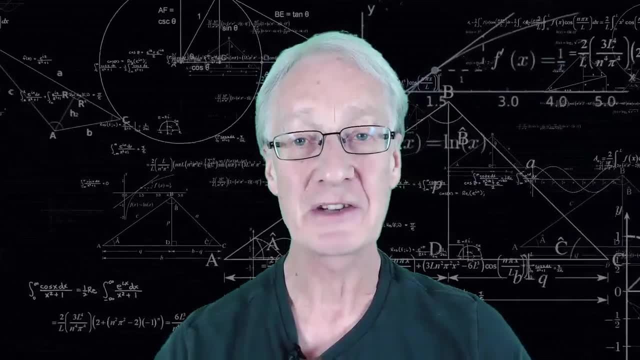 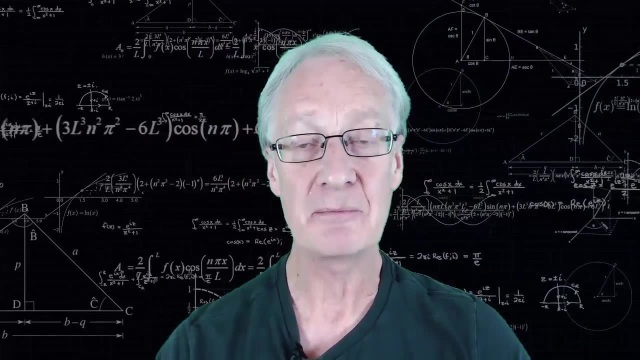 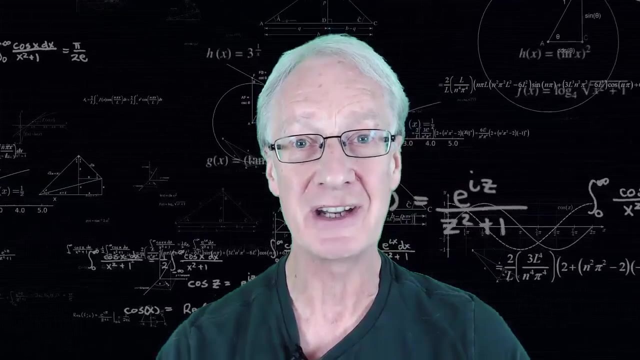 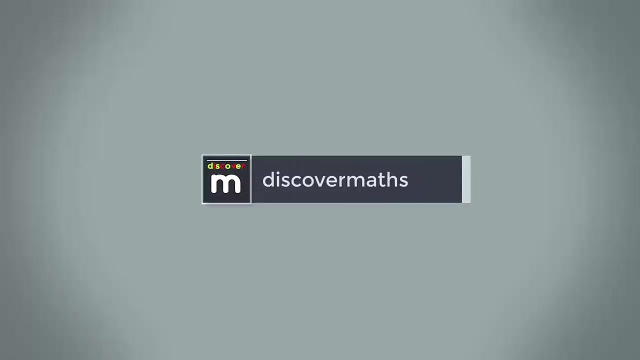 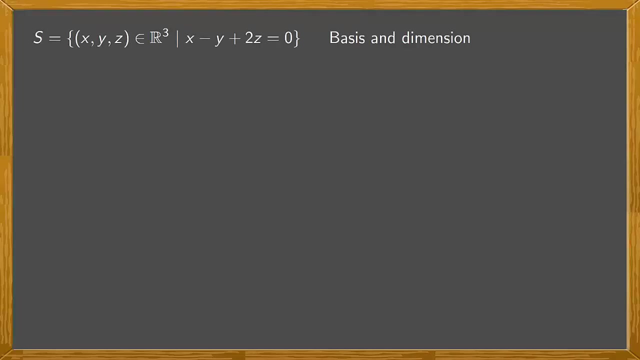 Hi again everyone. This is a video on vector spaces in which we're going to look at an example and calculate the basis and also the dimension of a subspace given by its Cartesian equation. Let's discover the maths. On the screen we have the subspace S. Now let's calculate the basis and the dimension. As you can see, the subspace is determined by a Cartesian equation. The vectors of S are x, y, z, such that when substituting them in the equation we get an equality. In other words, they're solutions of the system of equations formed by the Cartesian equation. So let's calculate the solutions. 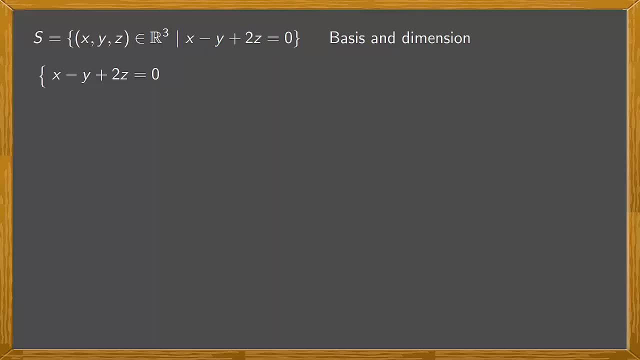 One way of solving a system of equations is Gaussian elimination, in which we carry out elementary operations on the equations. In our particular case, we have only one equation, so we can't reduce the system any further and we're ready to go Once the reduction is done. the number of parameters is equal to the number of unknowns less the number of equations. 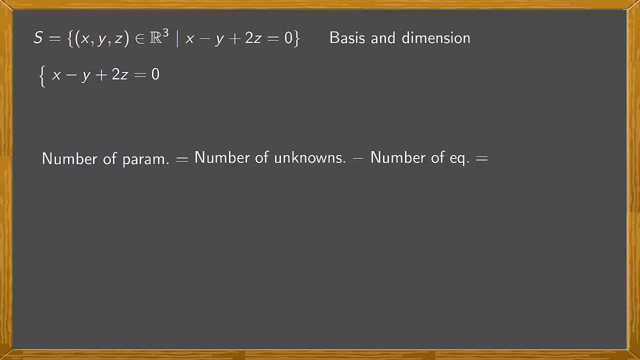 But we have to be careful because in the case of subspaces, it may be that some of the unknowns are less than the number of equations. The number of unknowns don't appear in the equations. In our case, the number of unknowns is 3 less the number of equations, which is 1, giving us 2 parameters. 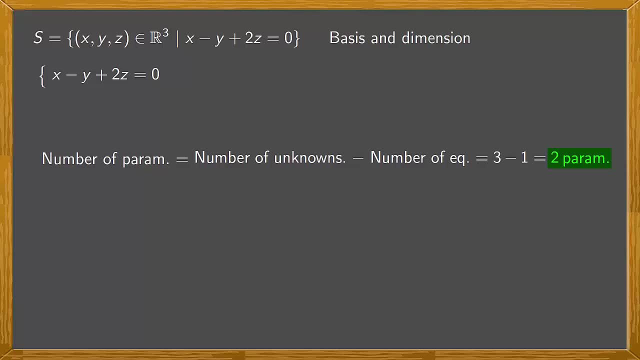 Now we have to assign the parameters to the unknowns. The usual way is to start at the end and if problems arise we'll find an alternative. In our case, let z equal alpha and y equal beta, where alpha and beta vary in R, Substituting in our equation, we have x minus y, which is beta, plus 2z, which is alpha. 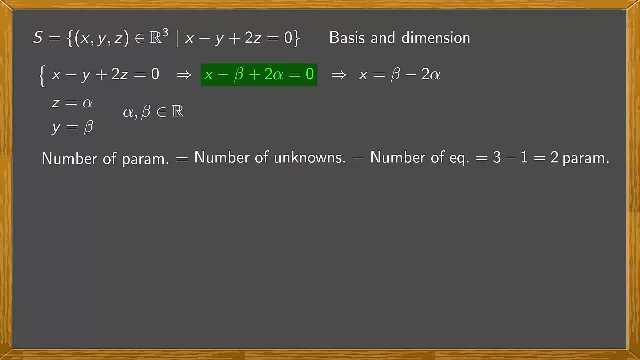 equals zero. From this we get that x equals beta minus 2 alpha. Now if x y z belongs to S, then x y z satisfies this equation. So it's a solution of the system and its elements have this form for certain alpha. 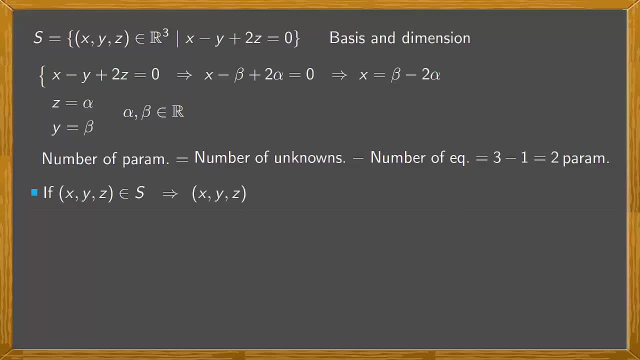 and beta values. Therefore, x, y, z equals x, which is beta minus 2 alpha, where y is beta and z is alpha. Now the trick is to separate this vector into a sum of vectors where only one parameter appears in each. 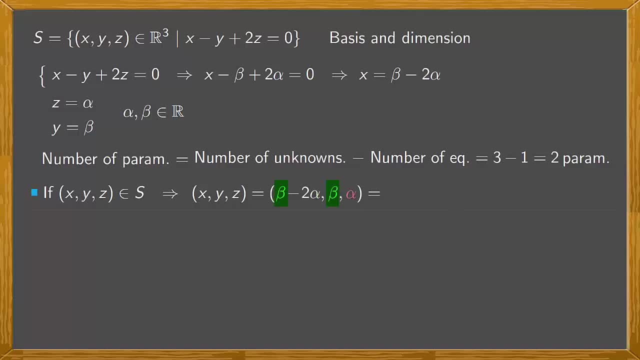 In our case a vector with only beta, beta, beta zero plus one with only alpha minus 2 alpha zero, alpha. Then we take out alpha and beta to give beta 1, 1, zero plus alpha minus 2, zero one. 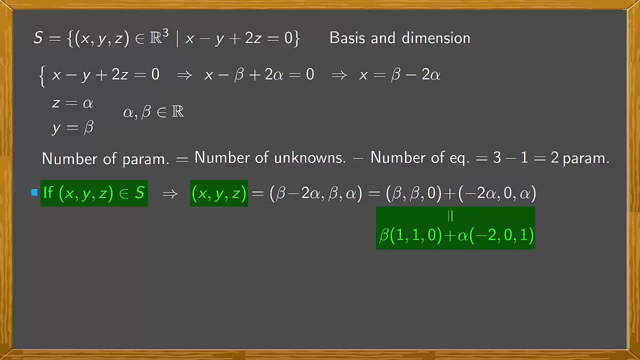 We've just obtained that every vector of S is a linear combination of these vectors, so that S is generated by 1, 1, zero and minus 2, zero one. So a generating system of S is the set 1, 1, zero minus 2, zero one. 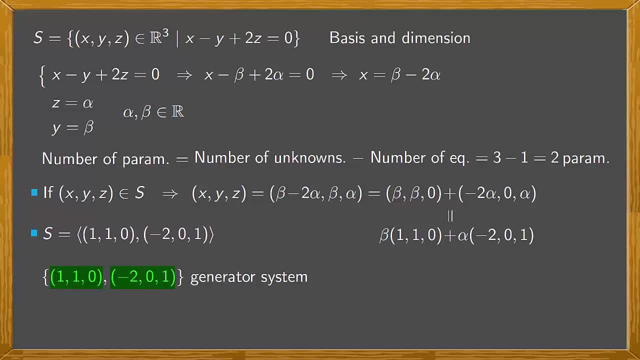 Notice that these two vectors aren't proportional, which means they're linearly independent. Therefore, this set of vectors is a generator system of S formed by linear combinations of vectors. They're linearly independent vectors and hence it's a base of S. 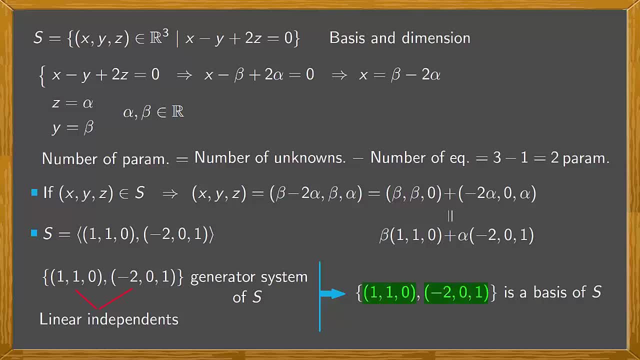 Also, as the base of S has two vectors, we have that the dimensions of S is 2.. Remember that all the bases of S will always be formed by two vectors. Before finishing, let's just mention that it's good to be able to detect errors, to 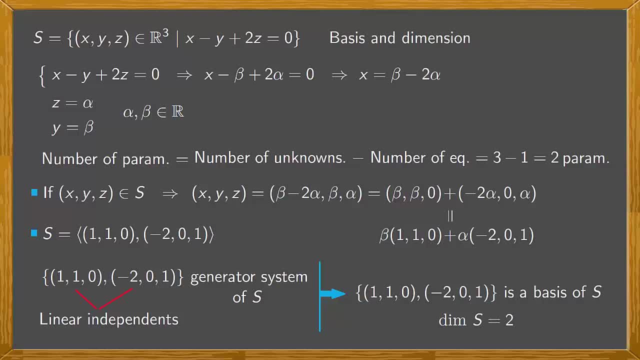 see if we've made a mistake along the way. For example, we could verify that the vectors of the base obtained are vectors of S, since otherwise we'd have done something wrong and we'd have to review the exercise. And if, for each of these vectors, you substitute components x, y, z in the equation of S, you 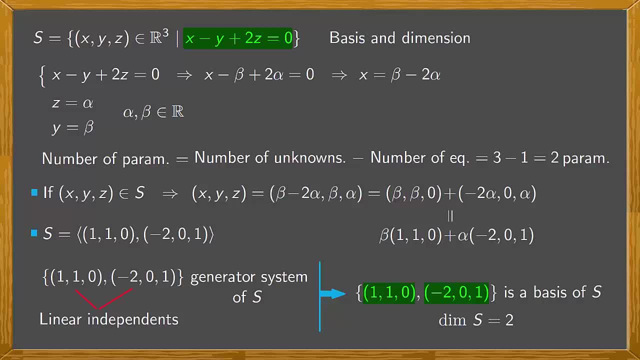 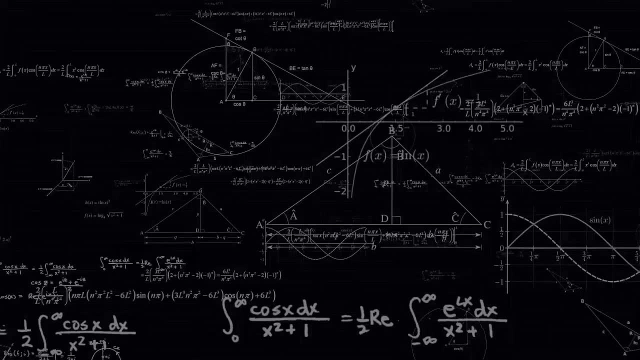 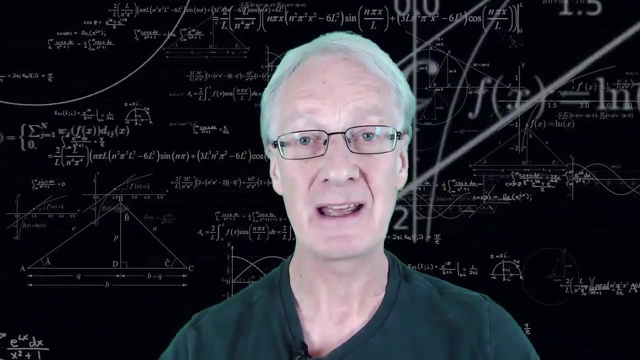 can easily see that the equality is fulfilled, so that these vectors are in S. It's a very good idea to do these checks at the end. Thanks for watching. I hope you found this useful, As usual. please subscribe if you haven't already, and I'll see you again very soon. to discover more maths.